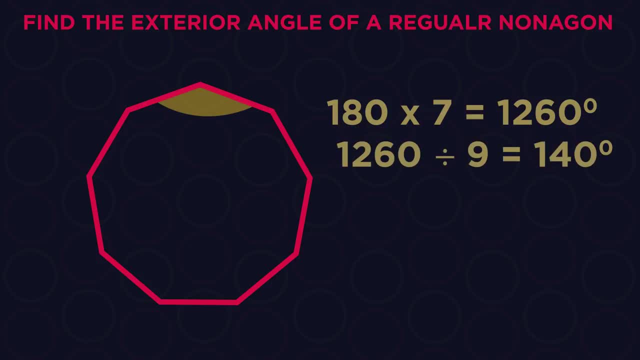 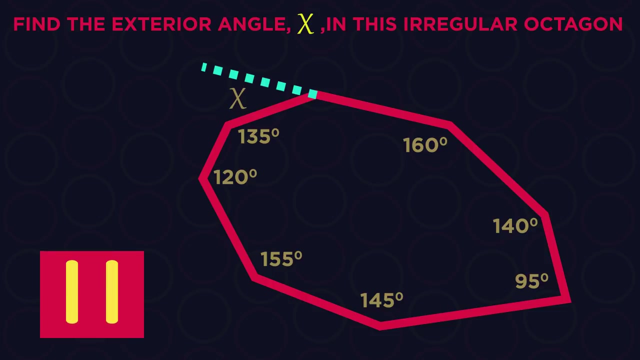 interior angle is 1260, divided by nine sides, which is a hundred and forty degrees. One hundred and eighty. take away one hundred and forty gives us the exterior angle of forty degrees. Simple, Here's one for you to do: Pause the video, find the angle and click play when you're ready. Did you get it? 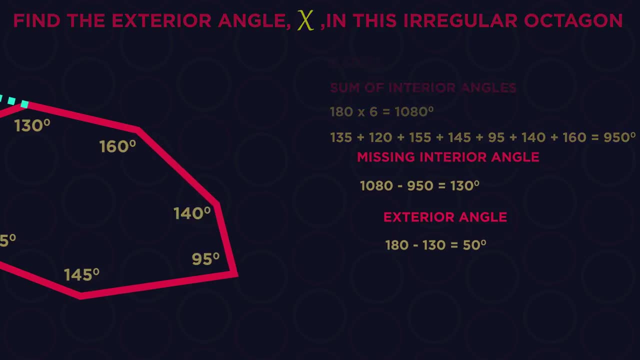 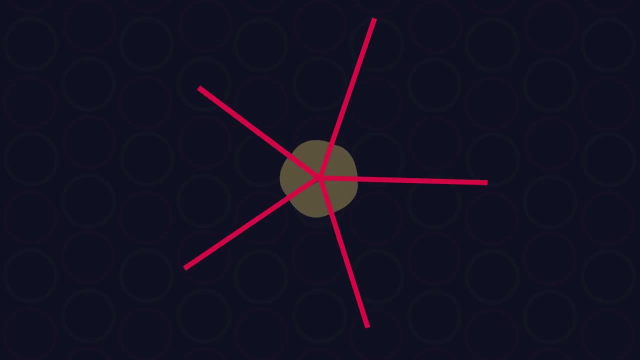 as fifty degrees. If we take all of the exterior angles and pull them together, they will always add up to three hundred and sixty degrees. This is true for any polygon. The exterior angles will always add up to three hundred and sixty degrees. This is actually really useful. We can use it to 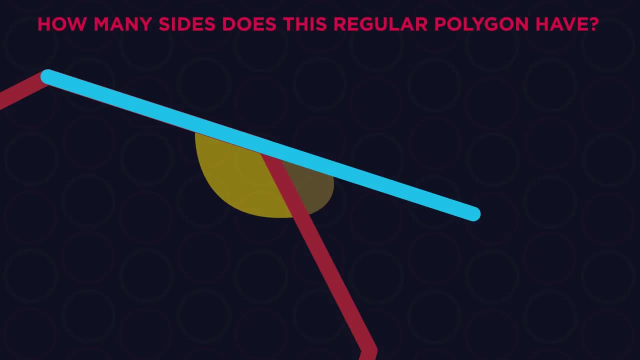 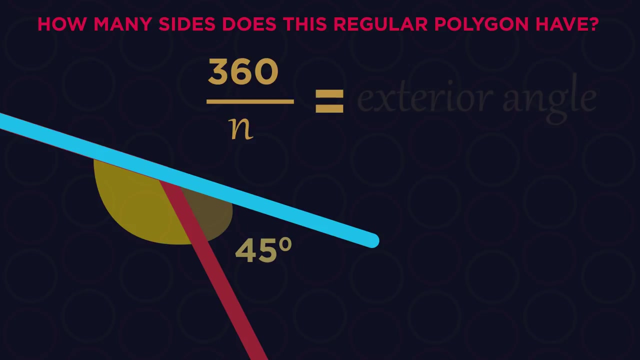 work out how many sides a regular polygon has. We're given the exterior angle of 45 degrees, As the exterior angles always add up to 65 degrees. 360 degrees will add up to 45 degrees. Soy thisine is 60. We know. 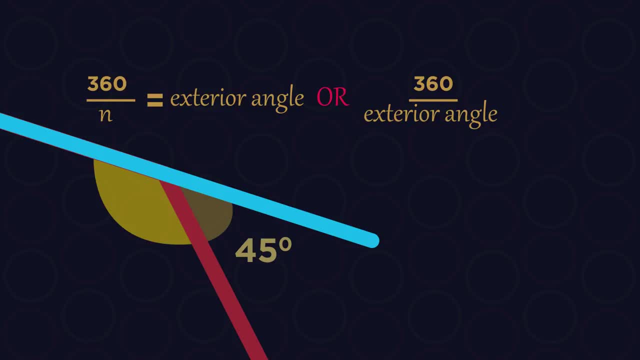 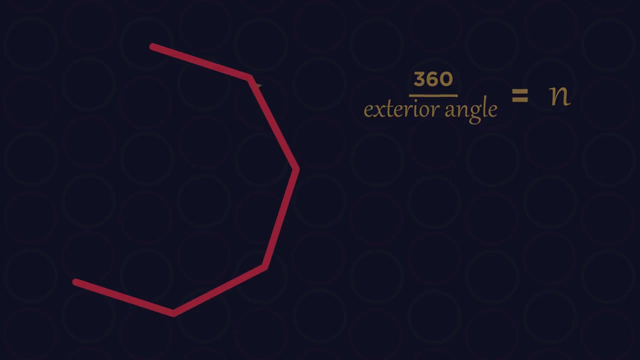 that 360 divided by the number of angles will equal the exterior angle. or simple rearranging: 360 divided by the exterior angle will give the number of sides. So 360 divided by 45 means this is an octagon. Here's one for you to do. how many sides does this regular prend? 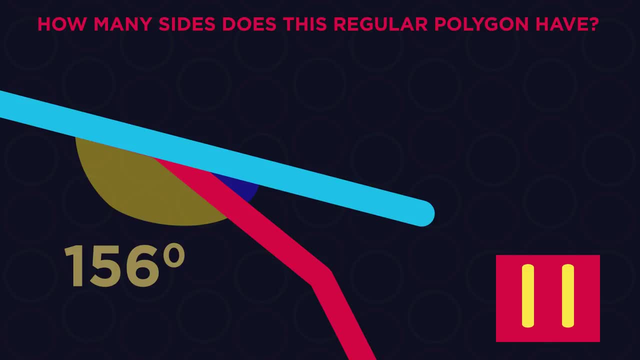 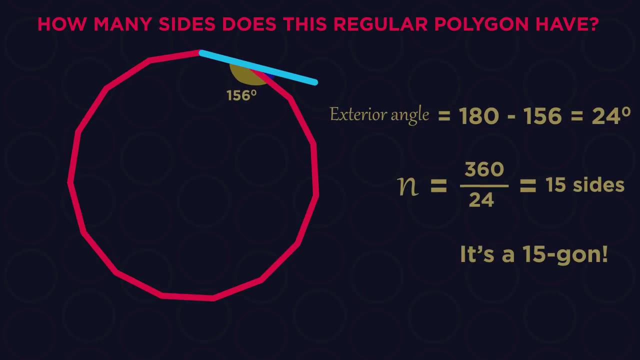 So I've typically put t訂ular τηςin a duplicated soиеfliero sìndoển veuxêtre. polygon. have pause the video, work it out and click play when you're ready. did you get it right? it's a 15 sided polygon. so there we have. finding the 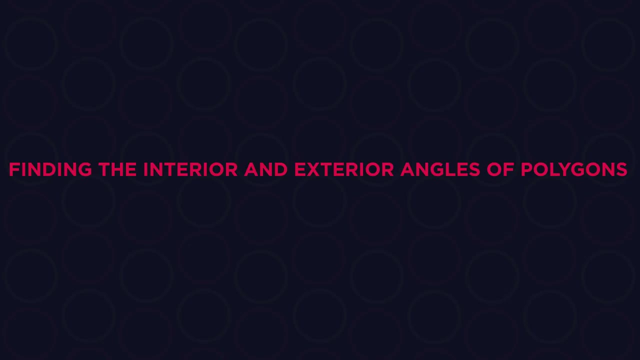 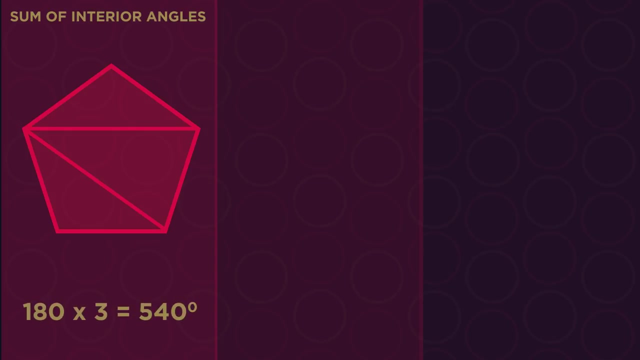 interior and exterior angles of polygons. for the sum of interior angles you subtract 2 from the number of sides and multiply it by 180. you can always fit 2 less triangles in exterior angles always make 180 degrees with the interior angle and exterior angles always add up to 360 degrees combining.